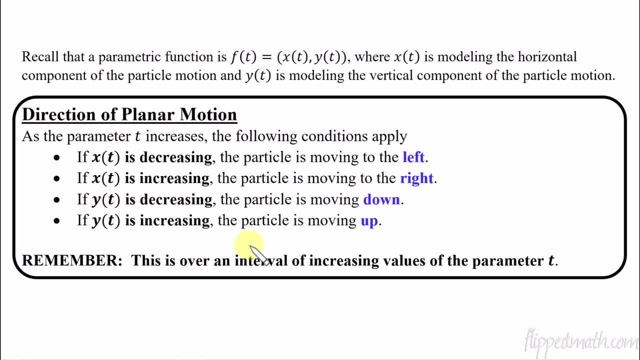 then we know the function is moving down, increasing, moving up. Okay, so kind of common sense there, but we want to make sure we put it into words And then we need to. oh, and we got to remember that this only is applying if we're increasing in t. 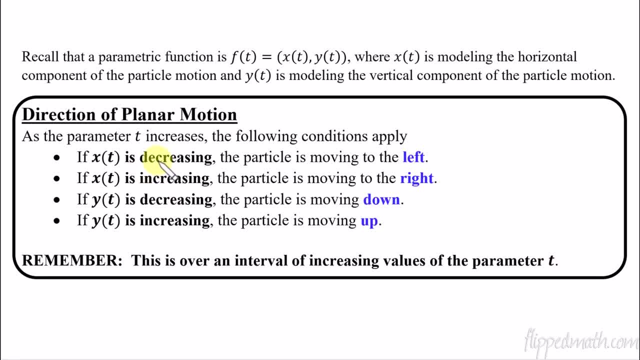 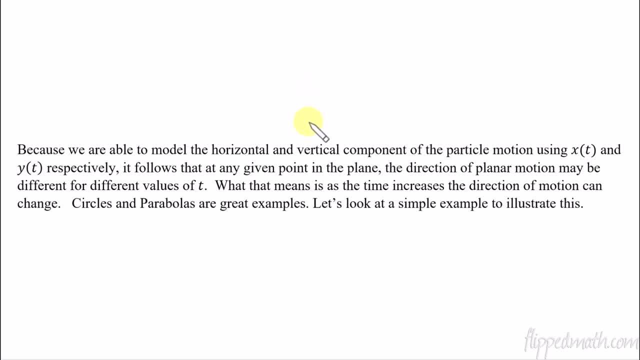 values right, The parameter has to be getting larger for us to be able to tell if x of t is increasing, decreasing, y of t increasing, decreasing. Now this little paragraph statement here. this is just to make sure that you know that this part here, that the planar motion, 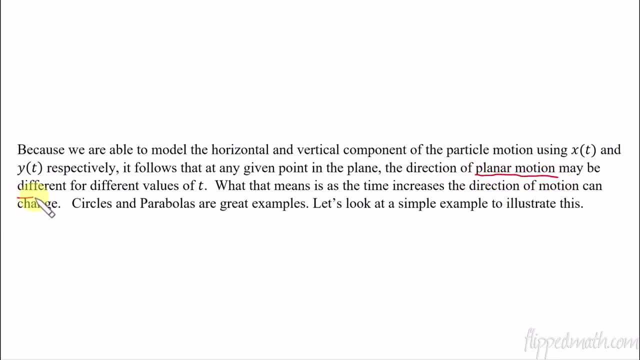 planar motion may be different, So the direction it's headed up, down, left right, any of those things are going to be different for different values of t, So it just kind of depends on what the function looks like As t changes. you could be going back and forth, In fact you might even. 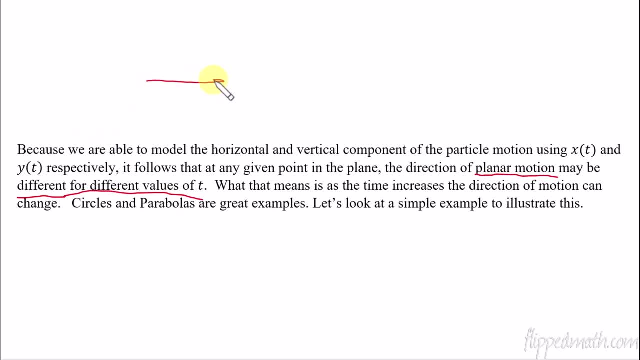 this is kind of cool. Sometimes you have this, you might have a line that goes like that, And then the graph just turns around and comes right back on the exact same line, And then it goes back on the exact same line like that's a possibility. So just it might be, go back and forth on top of. 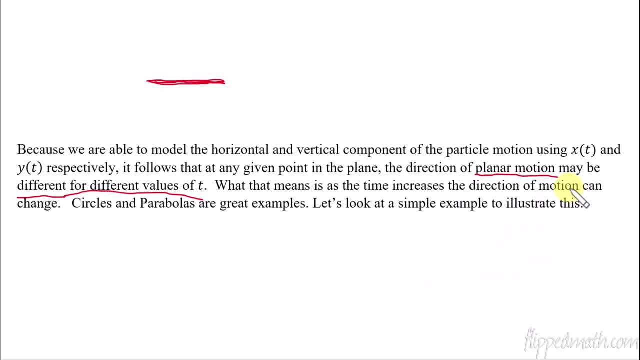 itself. It, just as time increases, the direction of the motion can also change. All right, so we're going to look at an example of a circle. circles, parabolas- those are great examples. So let's look at an example of a circle to show what we're talking about. We will do circles later in unit. 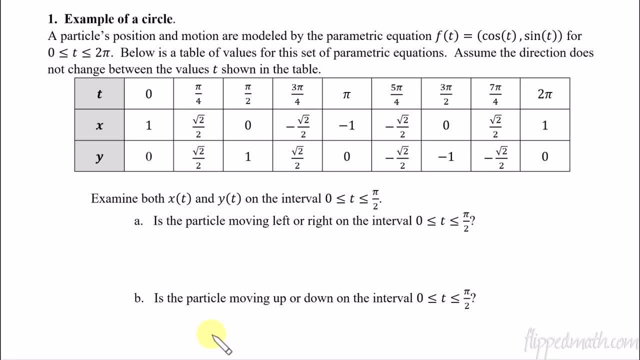 four. Okay, so this is- don't stress about how you're going to do circles later in unit four, How to create a circle or anything like that. This, I'm giving this to you. So here's an equation for a parametric equation: f of t equals cosine sine t. I already filled out the whole table, So 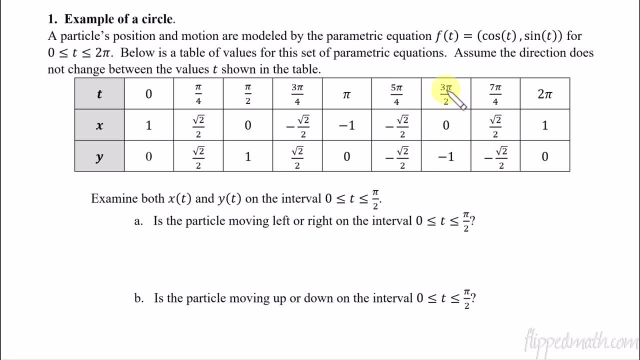 we don't need to deal with all that. I'll take all the time of that What? there is an important sentence in here. we're going to assume that the direction does not change between values of t, So it's going to only change at the values of t. So in between zero and pi over four, the thing x and y. 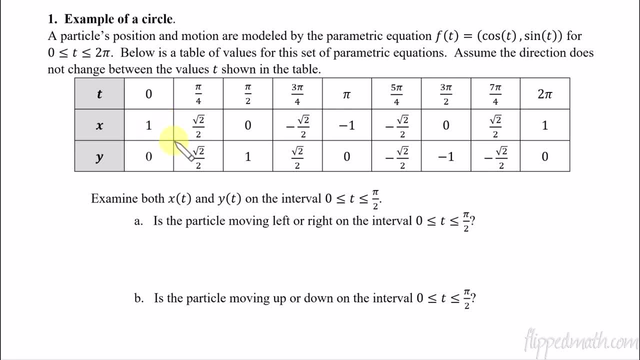 are going to either both be in or they're going to be either increasing or decreasing. You know it's not going to change in between there. That's an important thing, because if we didn't have the function and all we had was a table, you can't just assume that from this point. 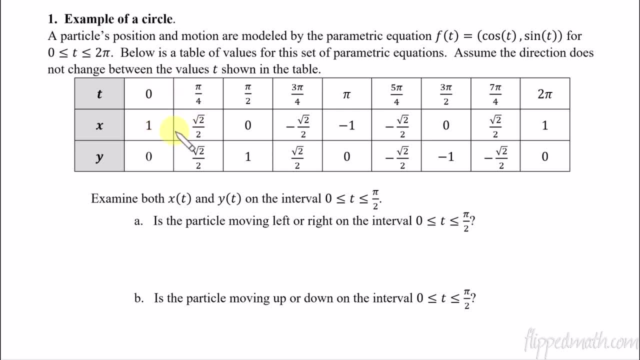 to this point that it's just increasing the whole time or decreasing the whole time. Okay, that is important. So this statement I've included just to make sure that mathematically it works out. We're going to keep these in this lesson really simple. Every time we have a table. 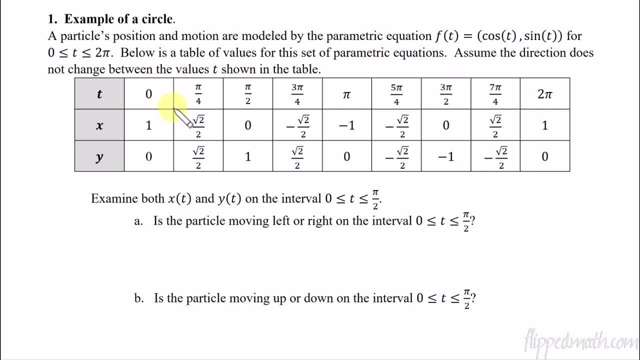 we're going to go ahead and just assume that the direction is not changing in between values. Okay, so I just want to make that statement real quick so that it's not throwing you off. All right. so the question is: is the particle moving left or right on the interval zero to pi? 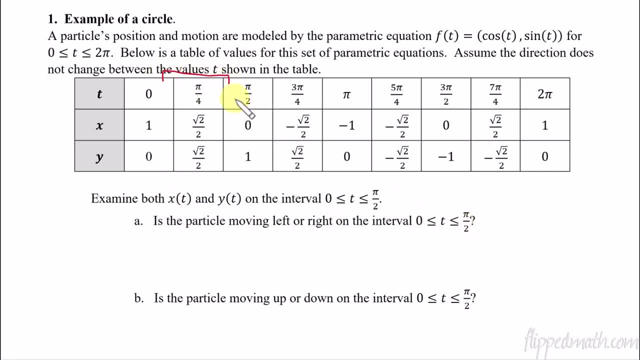 over four. So we're going to look at zero to pi or pi over two, excuse me, zero to pi over two On that interval, is it moving left or right? Well, left or right has to do with x values. right, That's an x value. So we're going to look here at this line and figure out if it's. 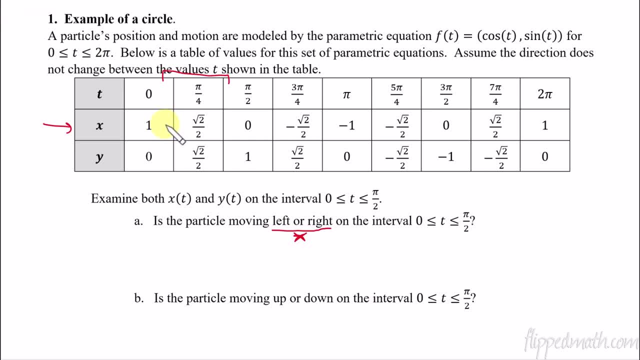 increasing or decreasing. So to get from here to here, what's the, what's this? the one value of one to the value of square root of two over two? Is that getting smaller or getting larger? You might not know. I mean, if you plugged it in the calculator you know this is actually going. 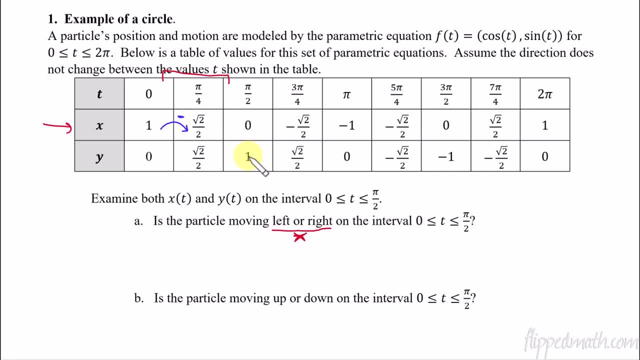 to be decreasing. I'm going to put a minus sign just to represent that it's decreasing. And then square root of two to two. that right there, square root of two, is also decreasing. So from zero to pi over two, it is decreasing. That means it is moving left. So the way we make that, 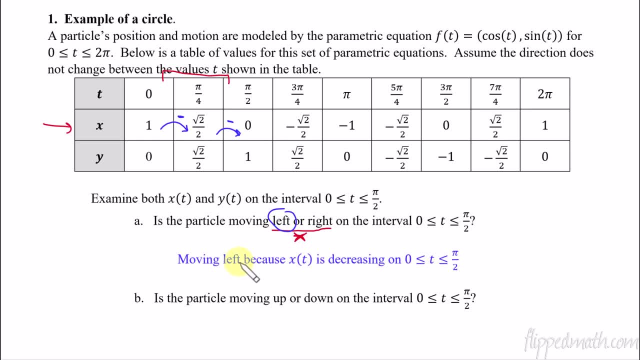 decreasing on the interval zero to pi over two. So this is the answer is moving left, And this is the justification of how we say, how we know that? because x of t is decreasing. All right, So now is the particle moving up or down? Same interval In order for it to be checking moving up or down. 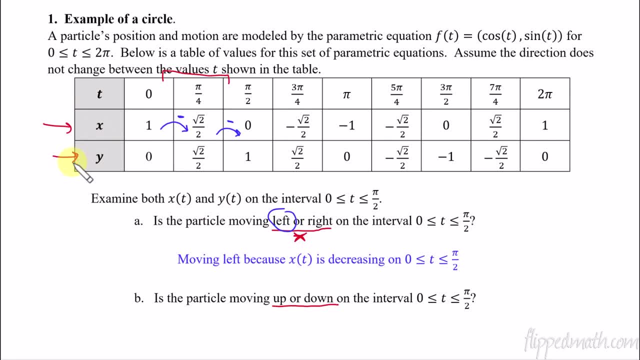 we're going to be looking specifically at the y values here. So then the y values from this goes from zero to square root of two over two. Well, that's obviously getting larger, So I'll put a plus symbol here. So it's increasing, And if it's increasing we've got to be moving up. So our 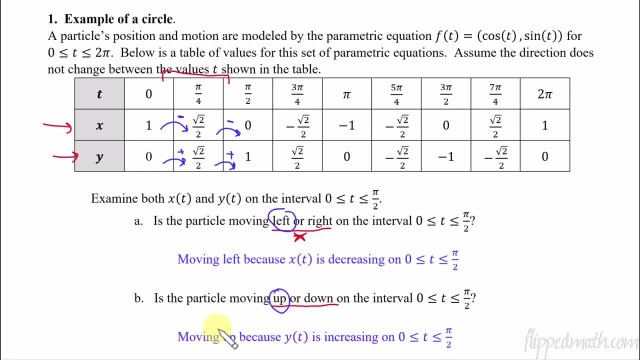 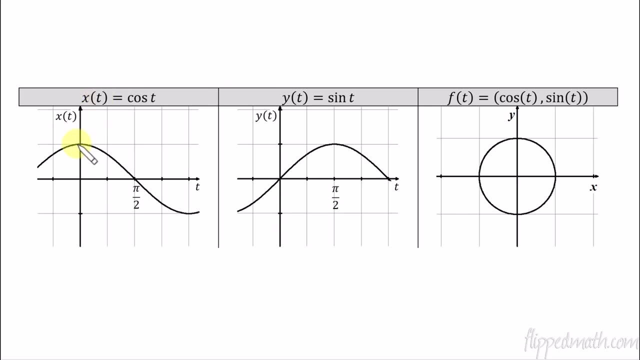 statement is moving up because y of t is increasing on that interval zero to pi over two Right now. I do have some grass below just to show what I was, what I'm doing here, So you can kind of get a feel for it. So this is x of t, x of t from zero to pi over two right here. That is decreasing. 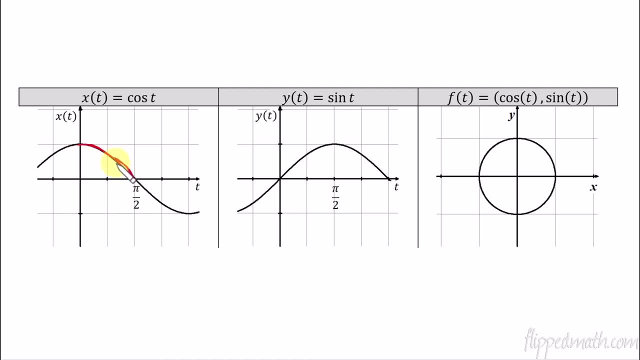 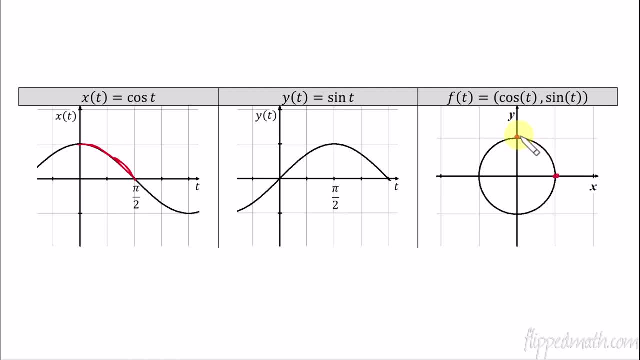 that means is that from zero to pi over two, the x values are decreasing. Therefore it must be moving to the left. That's supposed to be an error: flat arrow moving to the left. Okay, so that's what that's happening. from here to here, it is moving left. And then let me change colors here. 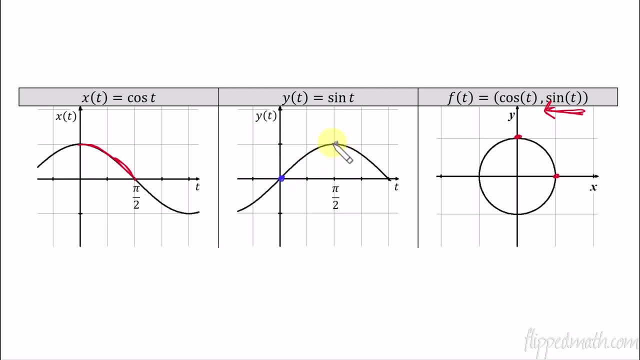 So sine from zero to pi over two is that function is increasing. Since it's increasing, that means the y component has to be going up. So from here to here the y component is going up. So yeah, that makes sense. This graph right here has the two. 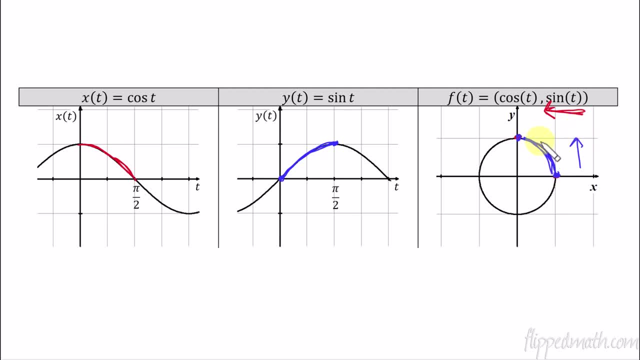 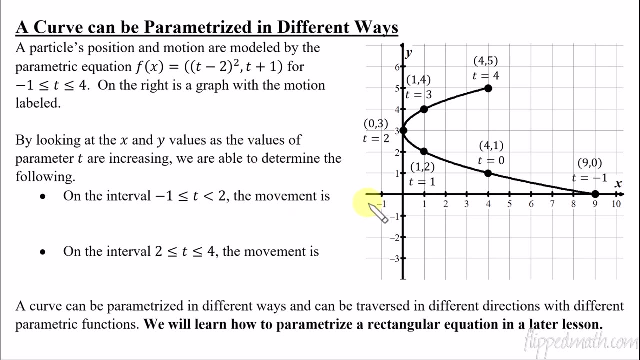 components of moving from here, from the left, from from- excuse me- moving left and moving up at the same time, And because of those two components we can see what's happening. This part of the lesson is just showing that you can have a curve and have different ways of writing it right. you can have 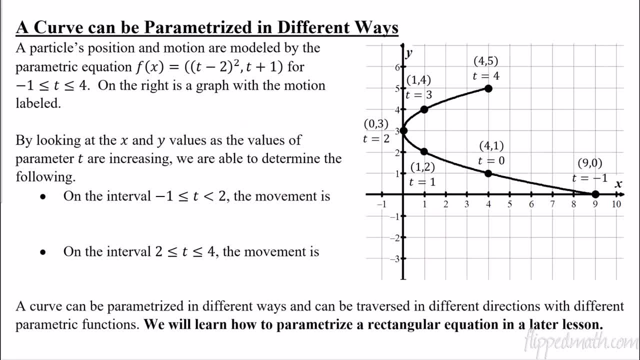 this parametric curve, But there's not just one, only one way of writing out a parametric function For that. So if we that's different for rectangular equations right for a rectangular equation. I mean, if you simplify the rectangular equation, it's the same rectangular equation every time. for that. 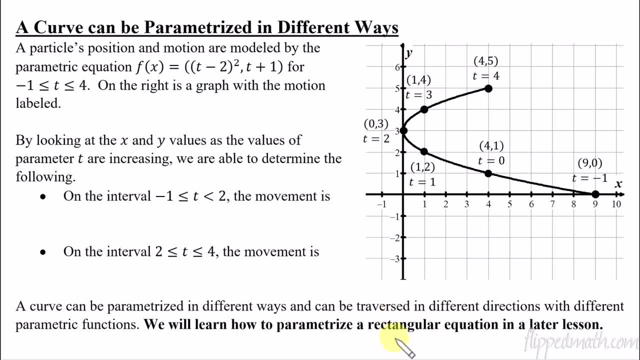 curve. you're not gonna have different ones Now. later on in this unit down here it says that later on in this unit, unit four, we're going to learn how to pair param, parametrize, parametrize- I don't know how to say this word- parametrize a rectangular equation. In other words, we're going 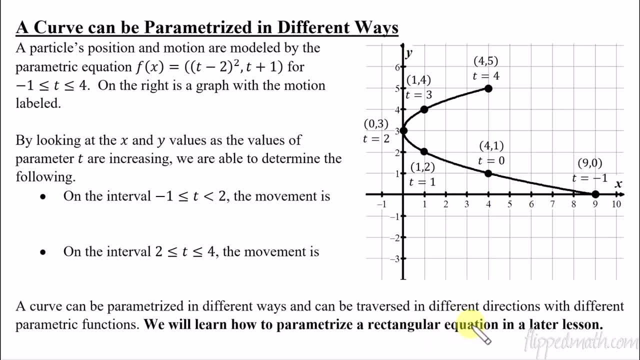 to learn how to take a rectangular equation and change it into a parametric equation. So we're going to learn how to do that in this lesson. I just want you to understand for this lesson that there's different ways of doing it. So here's an example of what we're looking at. We're not going to do a 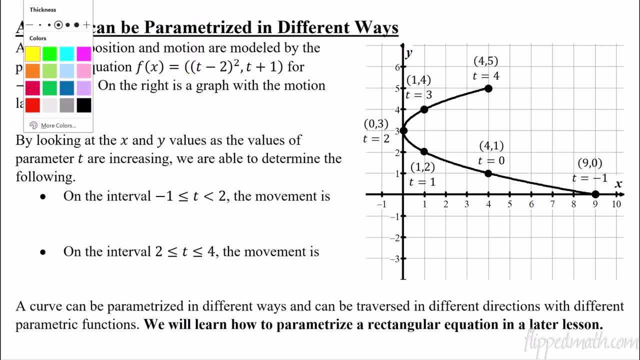 lot of a lot of calculations here. we're just going to look at some things that let me highlight: t equals one to t equals two. So we're going to start at negative one equals negative, one to t equals two. So, on that interval, what is the movement doing? So we're going to, we're going this direction. 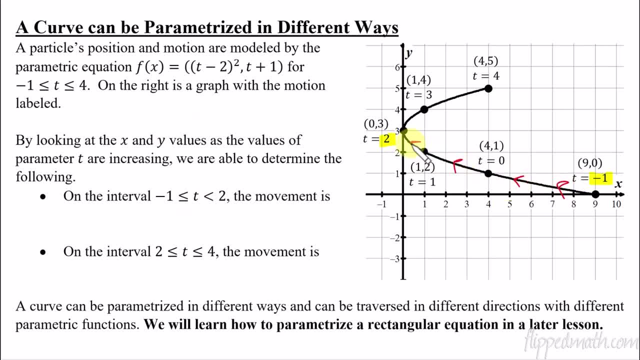 right. let's put some arrows down, Because the parameter t is increasing that way. So from t equals negative one to t equals two. the movement is left and up. we're moving left and up on that interval And then all of a sudden it changes direction And 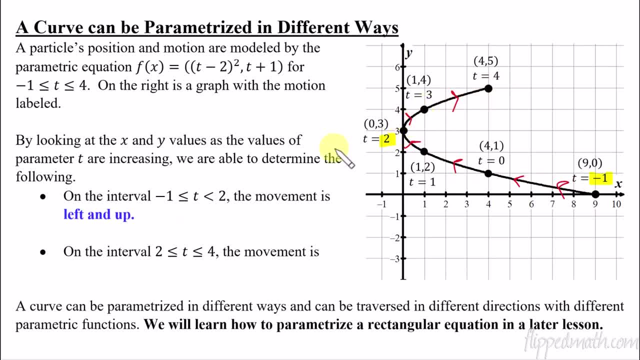 now we're going to go to the right and up on that interval. So, from two to four- there's my four right there On that interval- we're moving right and up. Okay, so pretty simple. That's all I wanted to show you on this one, Because now I want to show you that we can create exactly the same graph. But 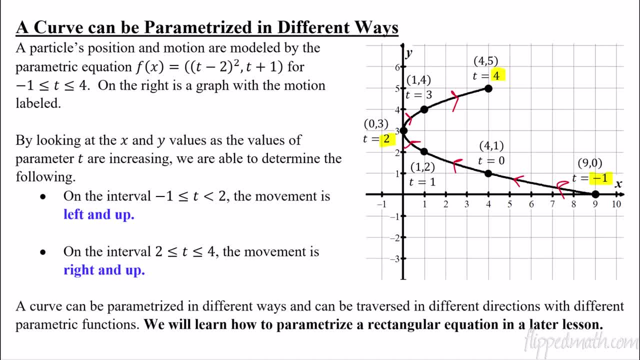 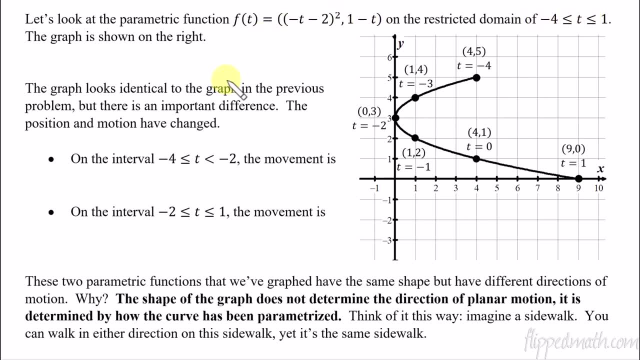 this time we're going to bring this graph to minus s. Let's say what was earlier: t minus two, quantity squared in t plus one. this is now going to change to negative t minus two and one minus t, and then the restricted domain is different. The graph is identical. It looks exactly the. 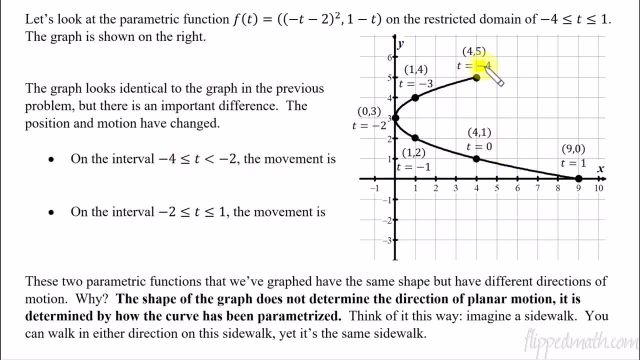 same. The difference is going to be the movement of the particle. So if I go from negative four to negative two, now I'm starting at negative four and going to negative two, And now the graph thing to show that this is the direction we're moving. now we're going to go down and to the 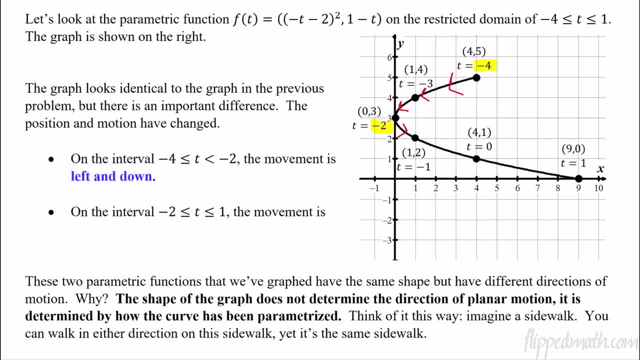 left, right, Yeah, Or left and down, if you want to say it that way. And then we keep going and we're going to go along this graph and now we're going down. this way It's turning, and now we're moving off to the right and we're going down. So we'd say that from negative two to a T value of 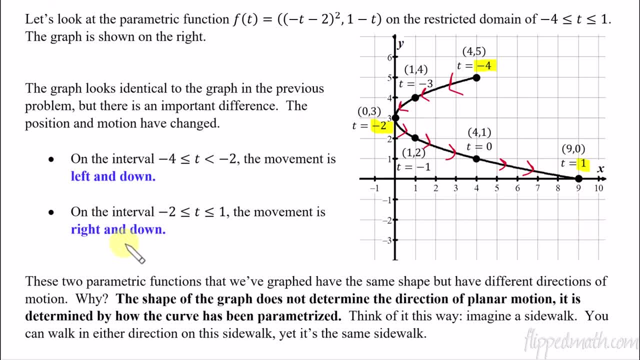 one. we're going from negative two to one We get. the graph is going right and down, All right. So the point of showing you that is that you have parametric functions that are different but give you exactly the same curve And you can just change. And if you change the parameter and change, 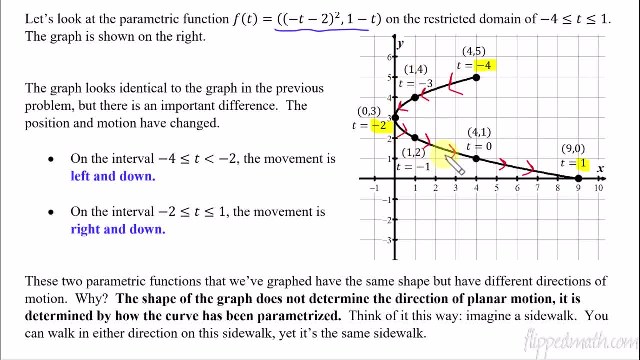 things around, you can actually make the motion go in a different direction. So that's the next part of our lesson. How can you just take a graph with motion and change the direction? get the exact same graph but change the direction. This is how we do that. So let's say you have X of T and Y of 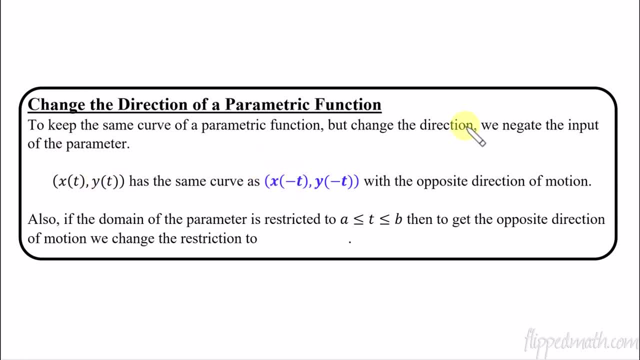 T, We're going to plug in a negative T. So that's what it is. We negate the input of the parameter. So instead of X of T and Y of T, you plug in negative T to both of, to all of the T values, And and then you get the direction of. 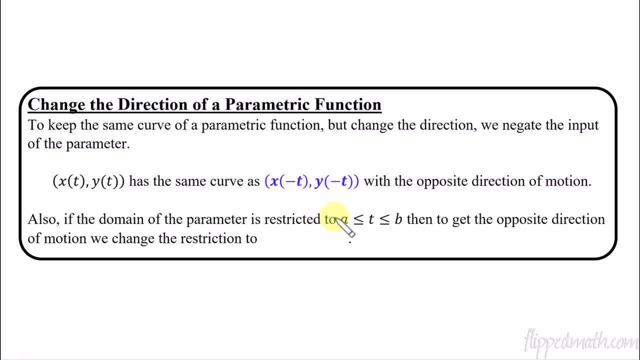 the opposite direction of motion. But if? if it's restricted, right, if the parameter is restricted, then we take the interval from a to B and we have to swap them. You're going to go from B to a instead and make them negative, So we're going from negative B to negative a. 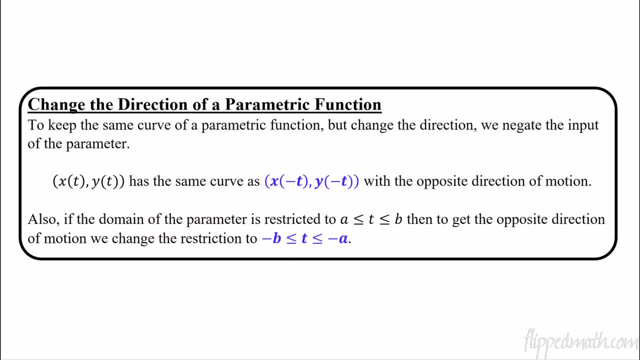 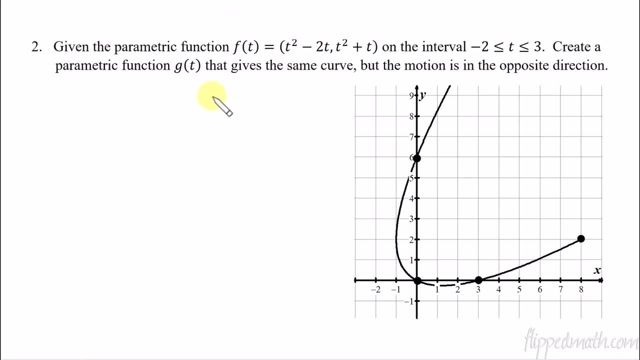 All right, That's how we change the direction. get a, get a parametric function like that. So let's, let's do a quick example of this. here We have a curve, This is the, this is the curve parametric equation, and we're starting off here and we're going this way. Okay, So just so you. 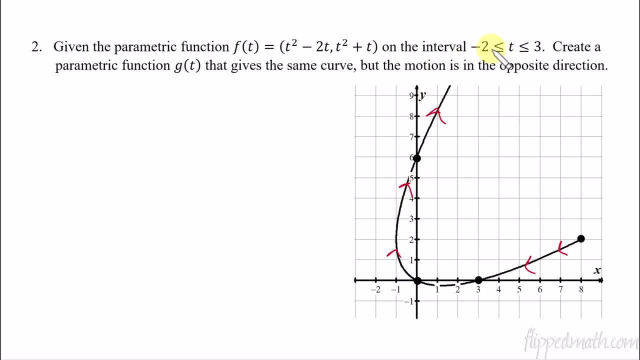 know that's the direction we're headed for this: from negative two to three. So this is starting at: T equals T equals negative two. So if we want to have exactly the same curve going the other direction, what we do is we take our X of T and instead of T we say negative T. So then you just 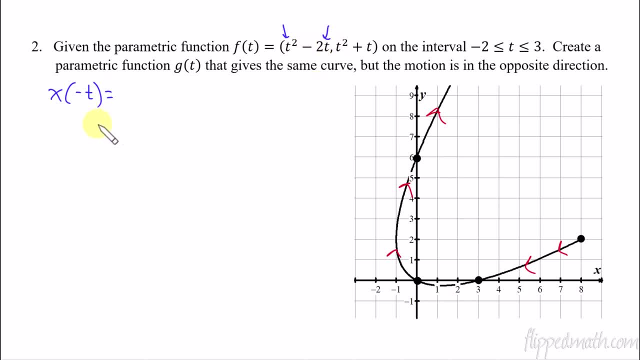 plug in a negative T into all the places where you see a T. So negative T squared minus two times negative T, not two T, And then that equals. simplify this out: We just get a positive T squared plus two T. So that's how that X component changes. Now let's do the Y. So the Y is going to. 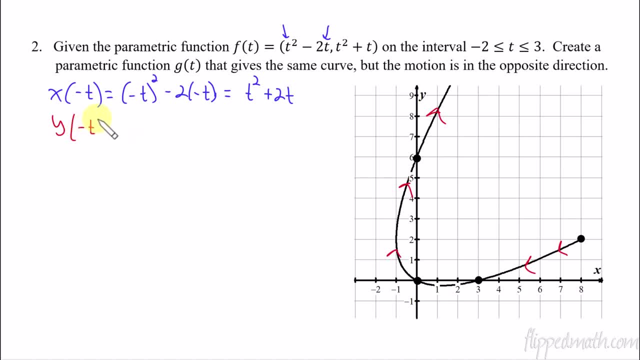 be T squared plus T, but we plug in a negative T that gives us negative T, quantity squared there negative T, And then, if we simplify that out, we get T squared minus T. So you can see, we've plugged in the T there and there the negative T, excuse me. So there's our new components of our. 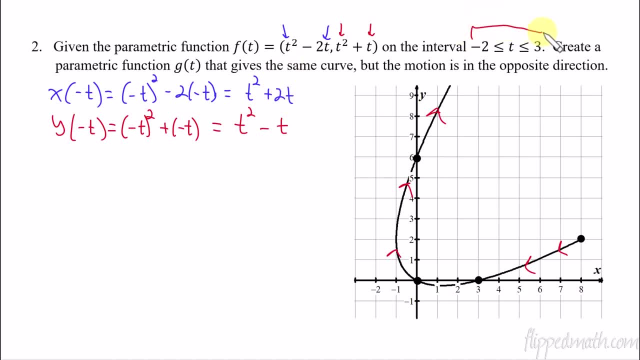 parametric function, And then we just have to figure out the intervals right. So it was going from negative two to three, And so now we're going to say on the interval: negative three less than or equal to, T less than or equal to, And then so we swapped the three and the negative. 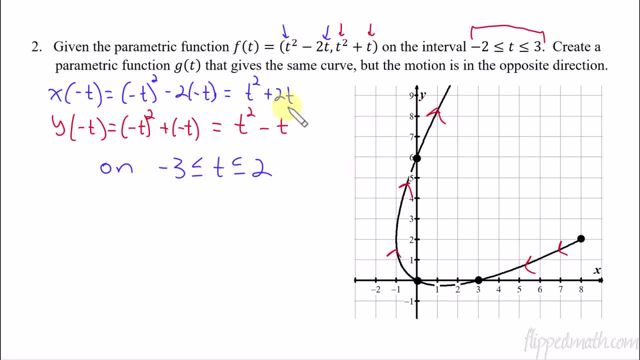 two and changed their sign to a positive two. So if we were to graph this right here, these are the components, the X component, the Y component, And then on that interval, you'd get the identical graph, but you'd be going. 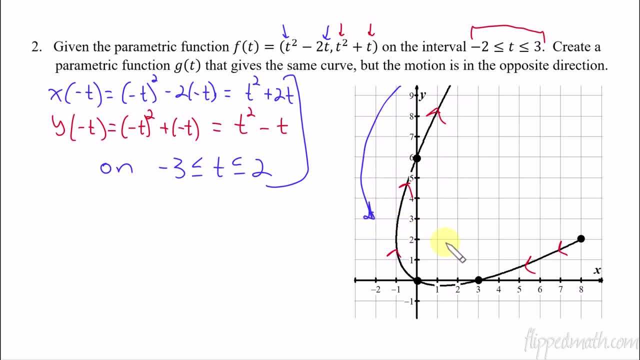 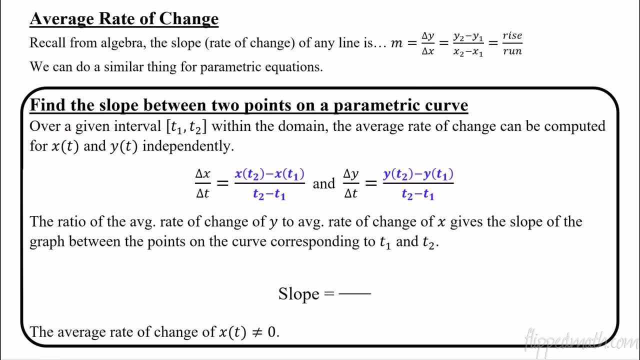 the other direction on this thing. So kind of cool how you do that. All right, last part of our lesson, And then we're all wrapped up, We're done here. That is the actual rate of change. So the mathematics behind this is pretty simple. The calculations, I should say, is pretty simple. 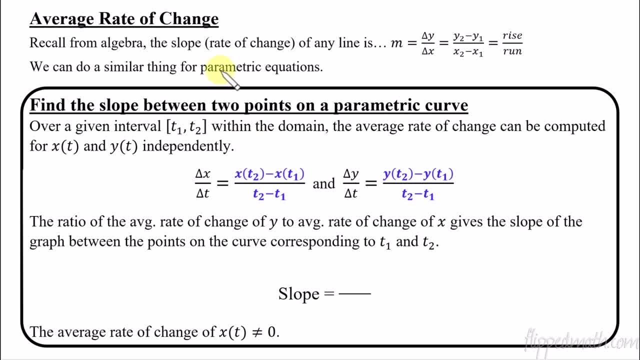 Remember, in algebra- even pre-algebra- you learned how to do the slope of a line, which is just the rate Change of the line. You would just have that the slope equals change in Y over change in X. Or you could think of this as Y2 minus Y1, X2 over X2 minus X1.. Or you could think of this as rise over run. 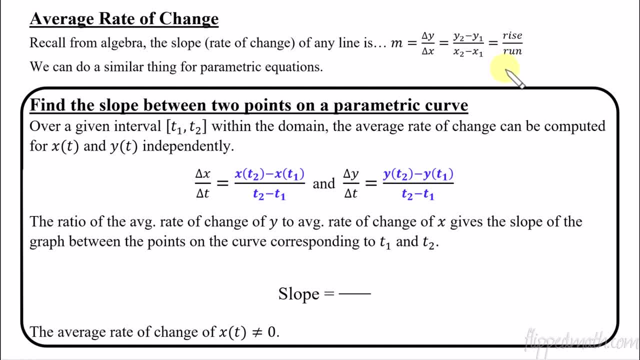 All the same thing here, right? So what we're going to do is a similar thing for parametrics, but you have to independently find the rate of change for X component and the rate of change for the Y component with respect to your time. So we're going to take two time values. We'll say: 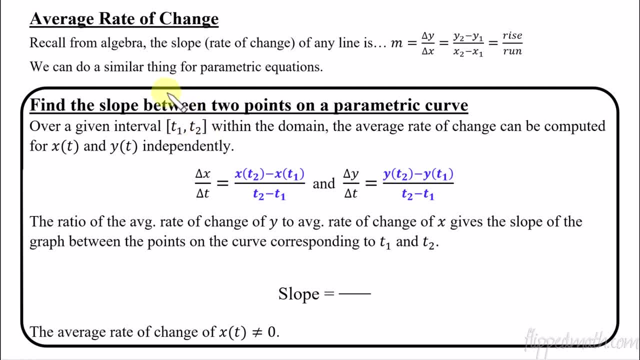 the first time value and the second time value, The parameter value. I should probably say So, those parameter values. we use those to find the rate of change for X and then the rate of change for Y. Once you have both of those, then you can. 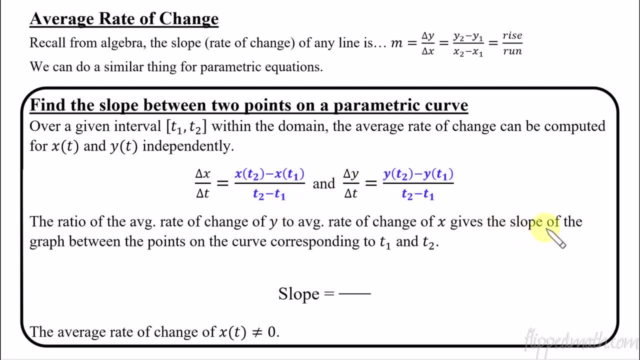 find the slope of the line. I'm going to change this. Your notes will say it gives the slope of the- I don't want to say graph, I know, I'm just being technical here- The slope of the line. It's going to be a straight line between two points if you connect it. So the slope of the line between: 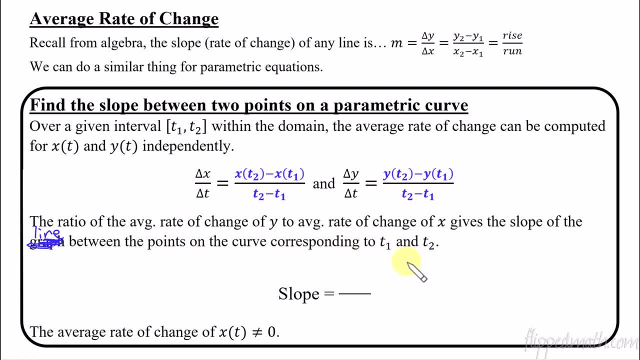 the points on the curve corresponding to T1 and T2 would be this thing: Change in Y over change in T, So the rate of change of Y divided by the rate of change of X. So it's still similar to this how you have change in Y over change in X, but you have to find the 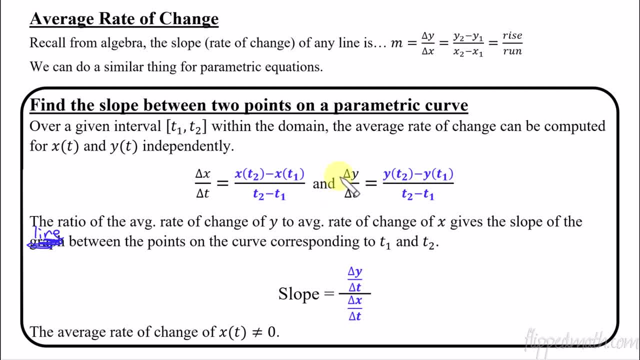 individual components. first, So each of those functions, you find the slope for those two points, for the two T values, And then with that you divide the two to get the slope of the line on a parametric curve, the slope of the line between two points. All right, Is that confusing? 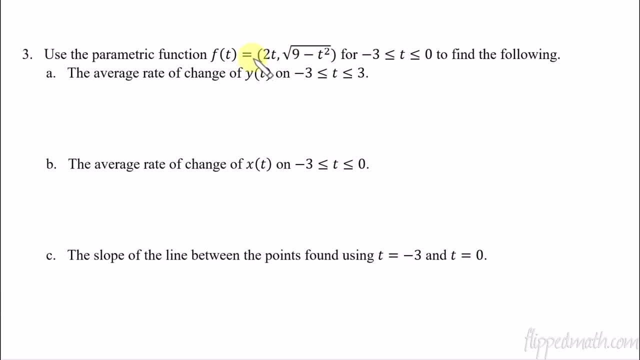 enough. Watch, It's not that hard. Let's do an example of this. So here we have a function and we've got the X component here, and you've got the Y component here, And we're only doing this on the interval of negative three to zero. Let's find, eventually, want to find, the slope of the line. 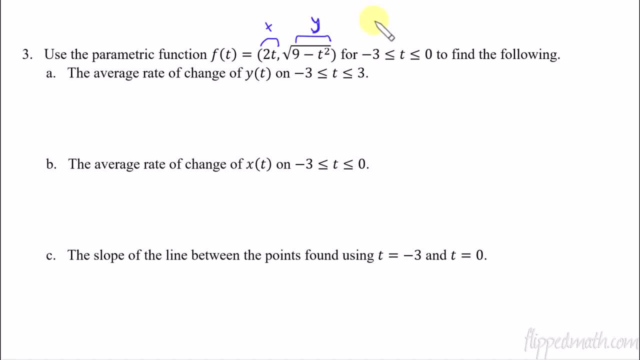 between the points negative three and zero. So we're going from negative three to zero. but we first have to individually find Y of T and X of T. So oh, that's supposed to be a zero right there. I will also fix that on your notes, Sorry. Negative three to zero. So we're going to 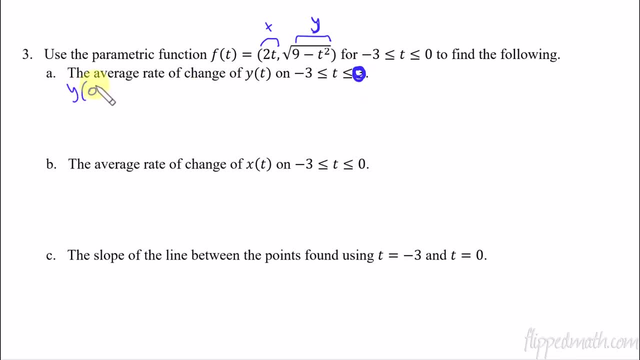 do Y of zero minus, Y of negative three. So then on bottom, if we started with the zero here, we got to do zero here minus, And then if we did negative three there, we got to do the negative three. You can. 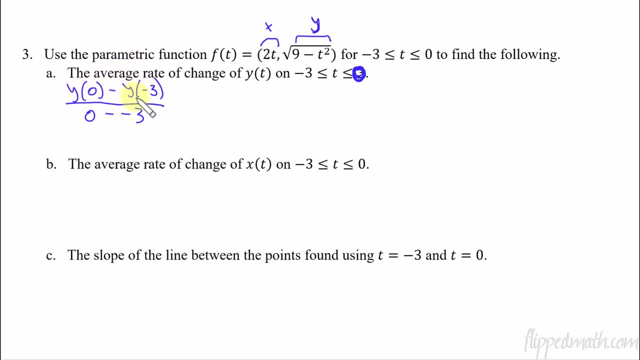 swap them right. You could do Y of negative, three first, if you wanted, minus Y of zero, but then you got to put them in the same order down here. Okay, Then we get equals. what's Y of zero? So this is where you might have to do some side work real quick here, Like: what is Y of zero? 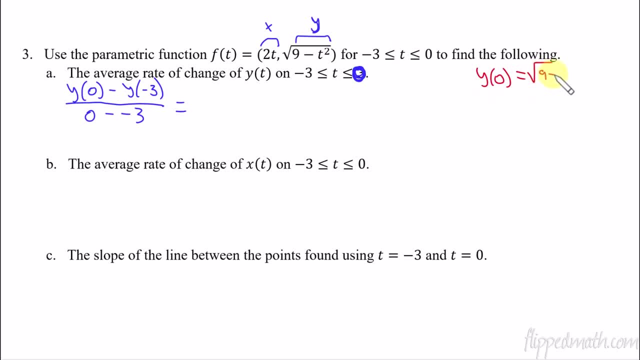 equal. Well, that's just the square root of nine minus zero. The square root of nine minus zero is going to be three. So then we can say: all right, well, then we're going to have three minus. And now we got to go: okay, well, what's Y of negative three? So you might have to do some side work to. 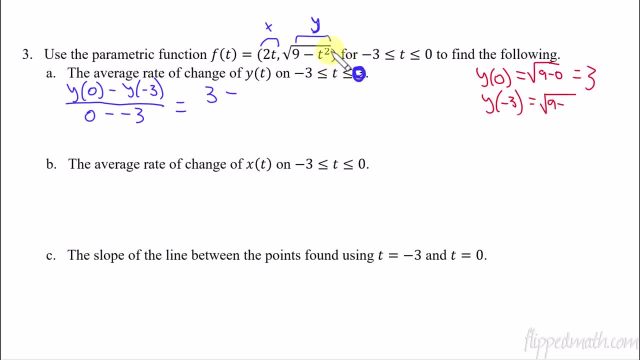 be able to figure these values out: Nine minus negative three squared is going to be nine and that equals zero. So we have three minus zero. on top and on bottom we have zero plus three. So we have three over three or just one. So the average rate of change is three over three. 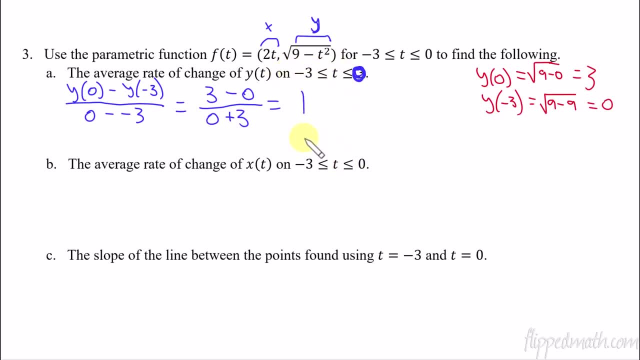 The average rate of change for the Y component from negative three to zero is one. All right, now let's find the X. So we got to do X of zero minus X of negative three. We're just doing very basic algebra skills here. Zero minus negative three equals. Now this one's a lot simpler.